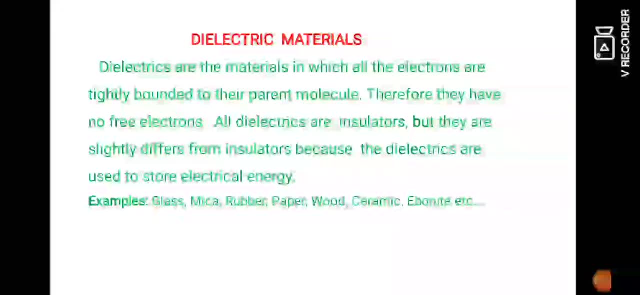 Metals conduct can conduct more heat or electricity than the insulating materials. The insulators are also having electrons. The conducting materials are also having electrons, But the insulators are not able to conduct heat or electricity. That is a difference between these two. 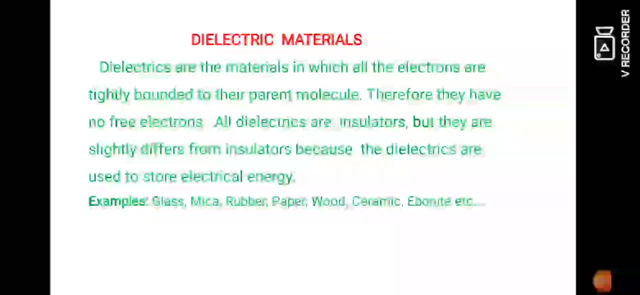 Because In the conducting materials, such as metals, the number of free electrons will be more. But in the case of insulators or dielectric materials there will be no such free electrons. Therefore they cannot conduct heat or electricity. So now let us see. what are these free electrons? 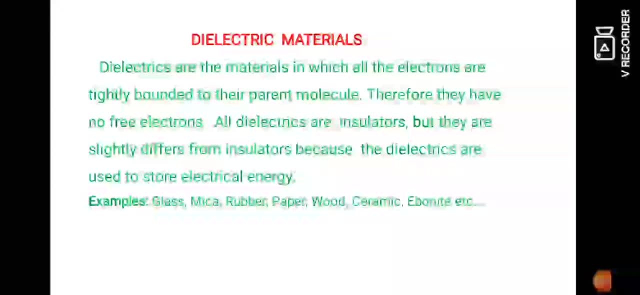 So the free electrons are nothing but the Electrons available in the outermost incomplete orbit of an atom. If the number of free electrons are more, The conductivity of the materials- Particularly the metals- will be more. If the number of free electrons will be less. 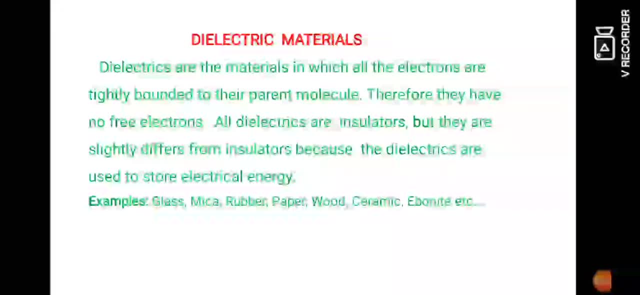 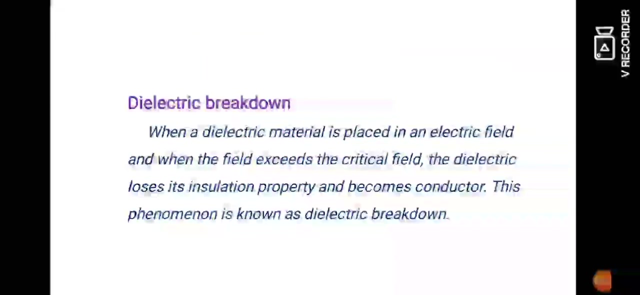 The conductivity of the material will also be less. This is a basic concept of The conducting materials And the Insulators Here. insulators are nothing but Dielectrics. Now let us see what is dielectric breakdown. We know. 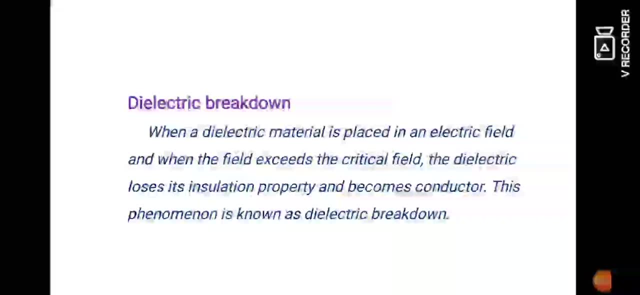 That the dielectric materials Are not able to conduct heat or electricity. Here we have to see what is dielectric breakdown. That means simply we can say: In some Circumstances The dielectric materials Will lose its Insulation property. 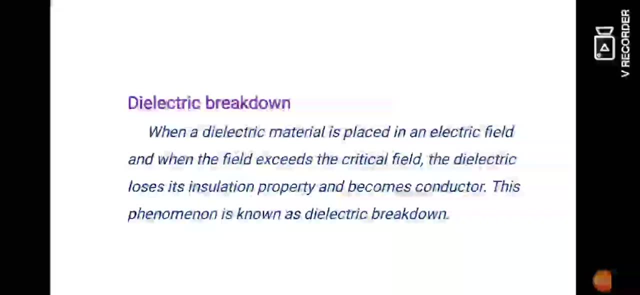 And suddenly becomes Conducting materials. This phenomenon is called as the dielectric breakdown. Now let us see What is dielectric breakdown: When a dielectric material is placed in an electrical field And when the field Exceeds a critical field value. 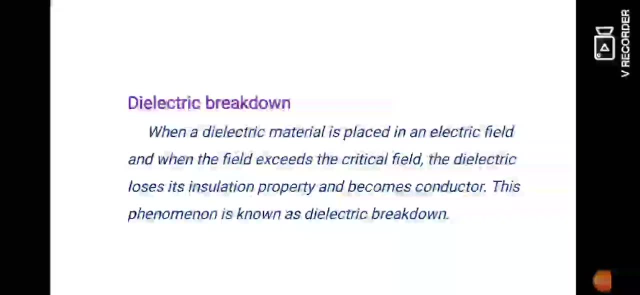 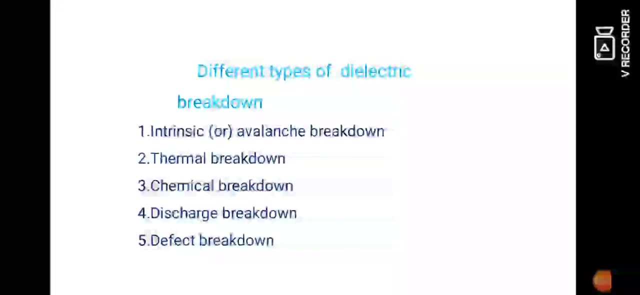 The dielectric Loses its insulation property And becomes conductor. This phenomenon is known as Dielectric Breakdown. Now let us see the different types of dielectric breakdown. The first one: Intrinsic or avalanche breakdown. The second one: 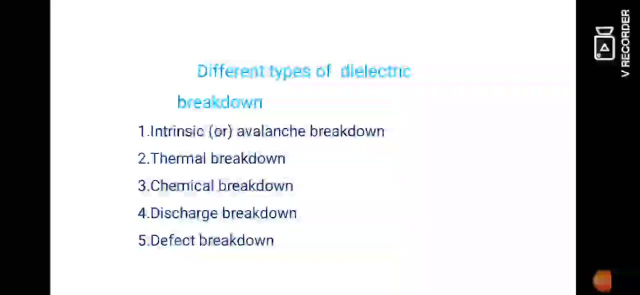 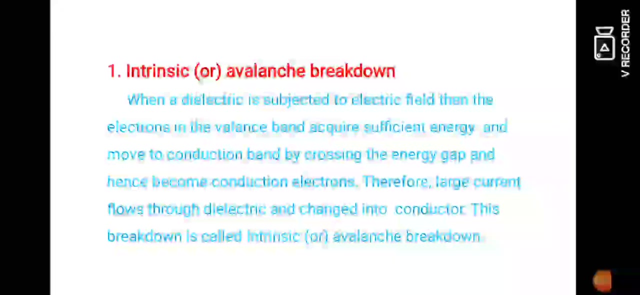 Thermal breakdown. Third one Chemical breakdown, Fourth one Discharge breakdown And the last one Defect breakdown. First let us see what is Intrinsic or avalanche breakdown When a dielectric material Is subjected to electric field. Then the electrons in the valence band. 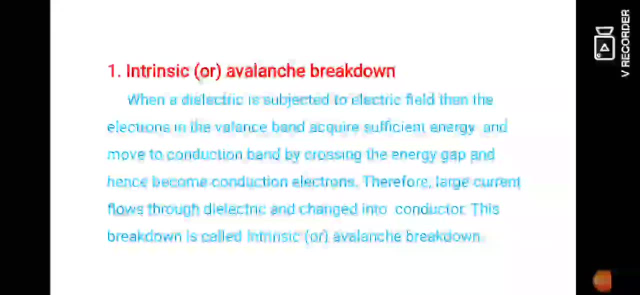 Acquire sufficient energy And move to the conduction band By crossing the energy gap And hence Become conduction electrons. Therefore, large current Flows through the dielectric And goes through the conductors And then Flows through the dielectric. 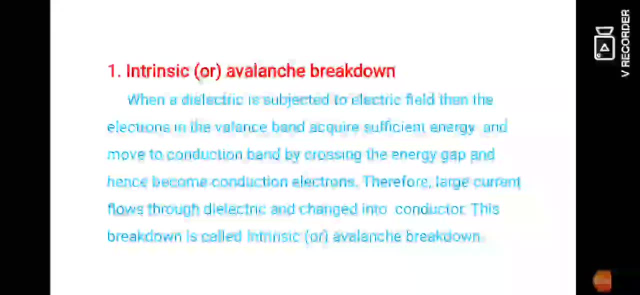 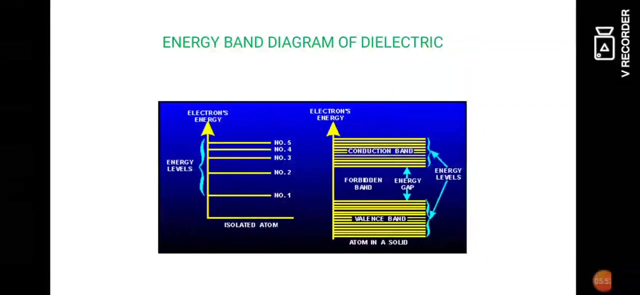 And changed into conductor. This breakdown is called Intrinsic or Avalanche breakdown. So this picture clearly shows The Intrinsic breakdown. We know That there are two important bonds. The first band is the Valence band, That is the bottom band. 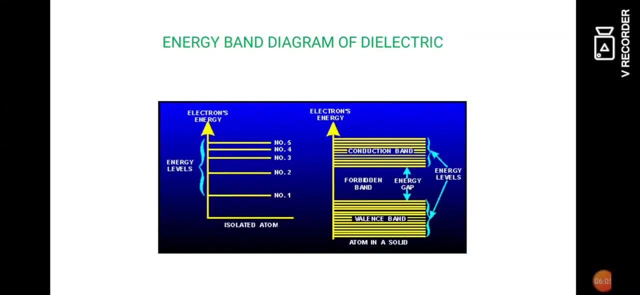 And the upper band is nothing But the conduction band. The Gap between these two Bands is called The forbidden band, Or energy gap, Since Few electrons are available In the valence band Of a dielectric When 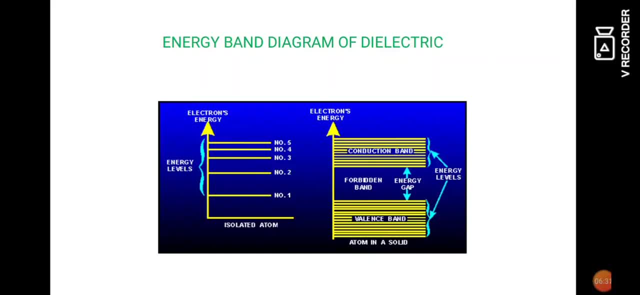 Huge quantity of Current is applied To this Dielectric material. These few valence electrons Will move from the valence band To the conduction band Through the Energy gap. As a result, When the electrons are moving, 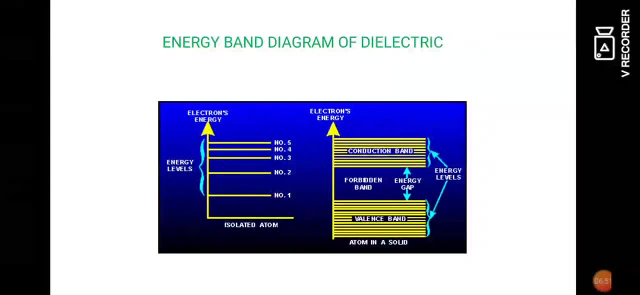 From the valence band To the conduction band The material Starts Conducting, So The dielectric will lose its Insulation property And it becomes the Conductor. So this is called as a Intrinsic. 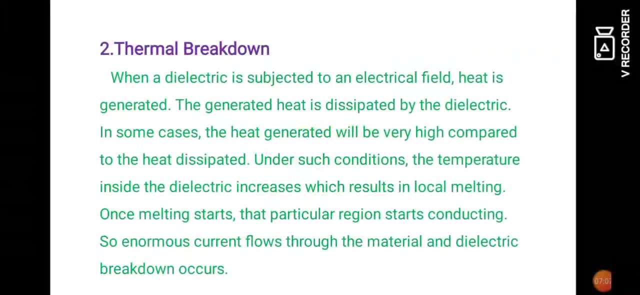 Breakdown. The second Breakdown Is Thermal Breakdown. Thermal Means Heat. When A dielectric Is subjected To an Electrical Field, Heat Is Generated. It is An Usual 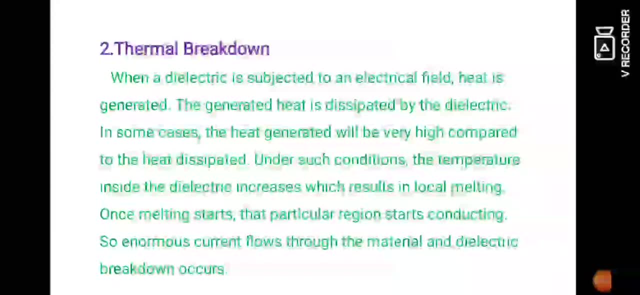 One. The Generated Heat Is Degenerated From The Dielectric, But In Some Cases The Heat Generated Will Be Very High Compared To The Heat Dissipated. 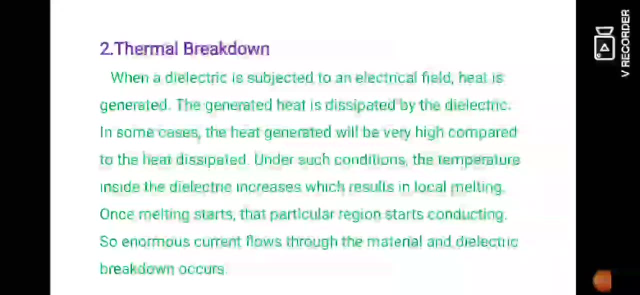 Dissipation Mean. The Heat Will Be Emitted In Any Weight. From Such Conditions, The Temperature Inside The Dielectric Increases, Which Results In Local Melting. 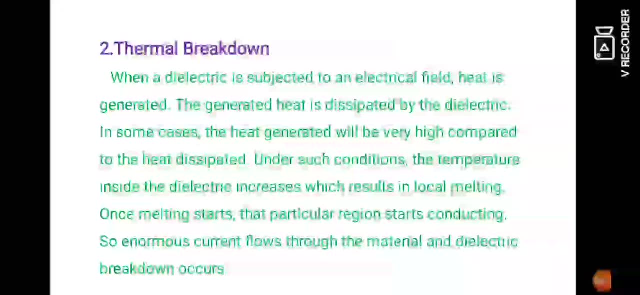 Of The Dielectric Material. Once Melting Starts, That Particular Region Starts Conducting In The Dielectric Material Breakdown Occurs. That Means The Area. 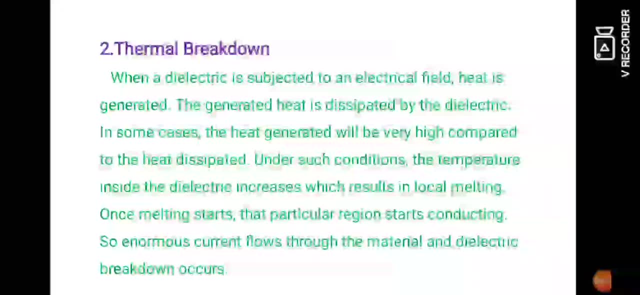 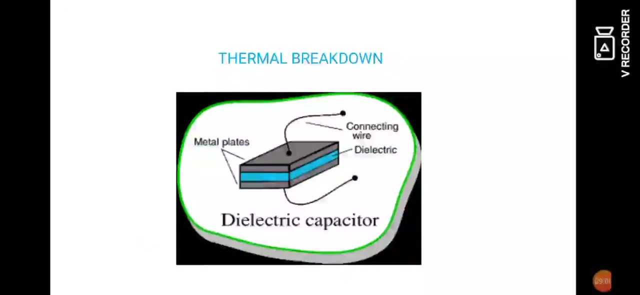 Which Starts Melting, Conducting The Electricity Or Heat That Is Due To The Heat Developed Inside The Dielectric Material. Therefore, This Type Now Let 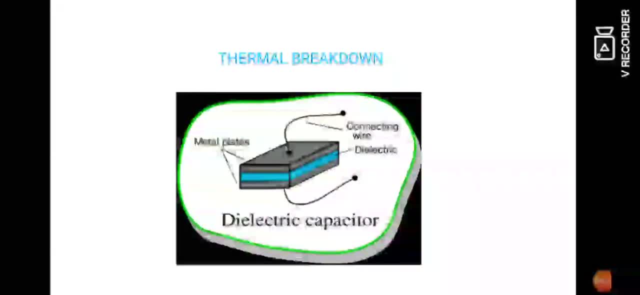 Us See The Figure Of Thermal Breakdown. Here We Have To Consider The Dielectric Material, Dielectric Capacitor, When Huge Quantity Of Current Is Flowing. 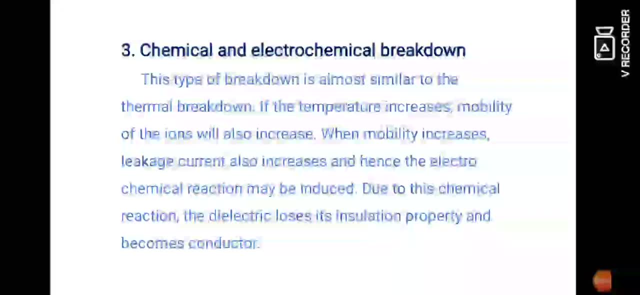 Through This Dielectric And Electrochemical Breakdown. So This Type Of Breakdown Is Almost Similar To That Thermal Breakdown. If The Temperature Increases, Mobility 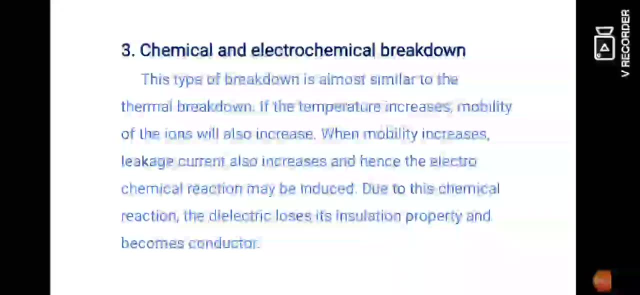 Of The Ions Will Also Increase. Mobility Means The Electrochemical Reaction May Be Induced. Due To This Chemical Reaction, The Dielectric Loses Its. 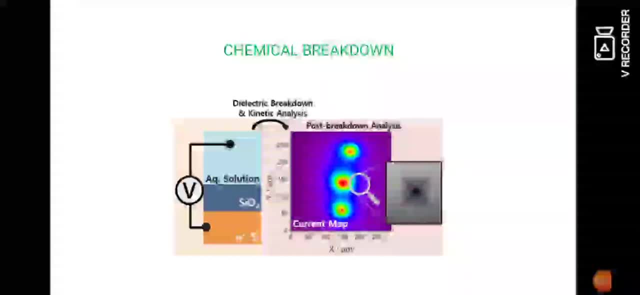 Insulation Property And Becomes Conductor. Now Let Us See The Figure Suppose When A Stability Of Ions In The Dielectric Material Will Be. 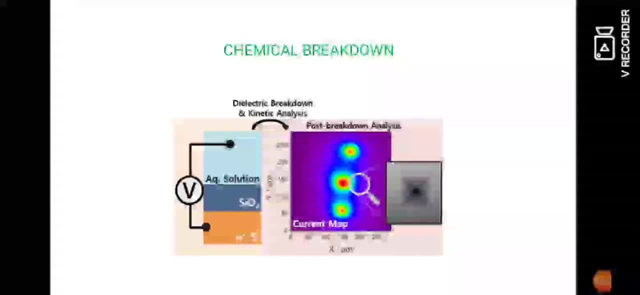 Increased, So That Its Energy Will Be Increased. As A Result, The Dielectric Material Starts Conducting Because Of The Decrease. Now Let Us See. 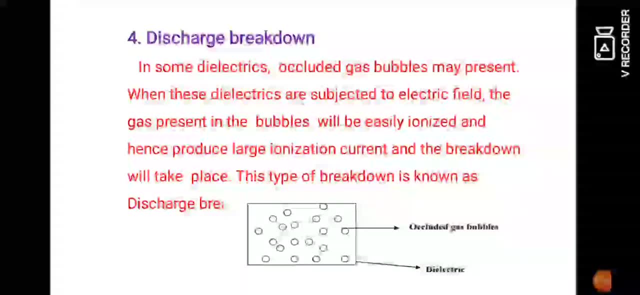 The Discharge Breakdown In Some Dielectrics. Accluded Gas Bubbles May Present. Accluded Means Very Dirty Gas Bubbles When These Dielectrics Are. 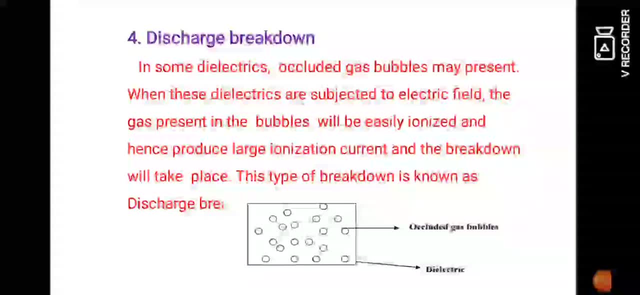 Subjected To Electric Field, The Current And The Breakdown Will Take Place. This Type Of Breakdown Is Known As Discharge Breakdown. This Is 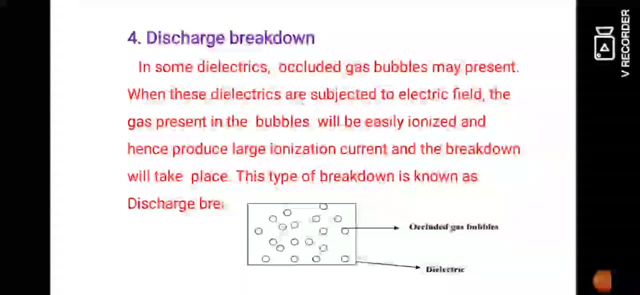 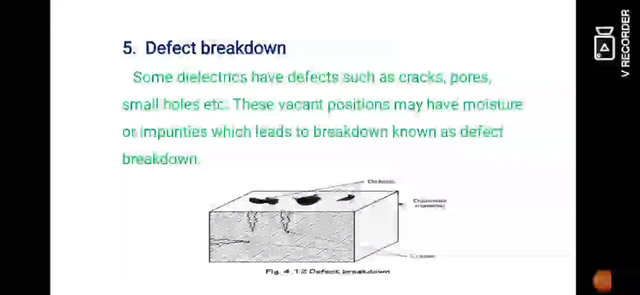 Mainly Occurred During Manufacturing Of The Dielectric Materials, So That Sometimes Due To Defects. Now Let Us See The Last Breakdown, That Is: 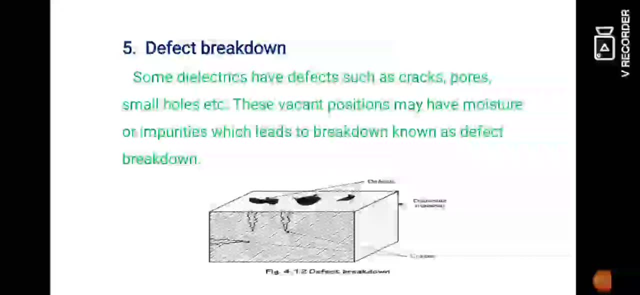 Defect Breakdown, Some Dielectric Have Defects Such As Cracks, Pores And Small Holes, Etc. All These Will Occur For Impurities.